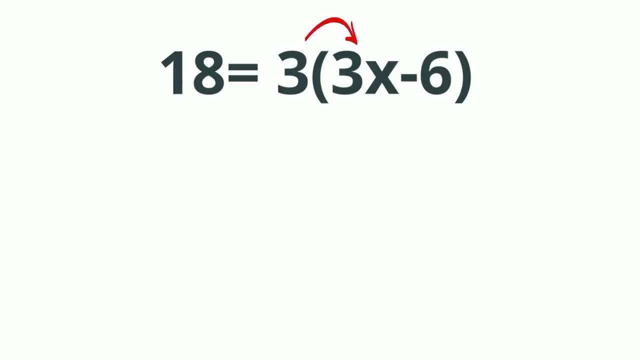 other. But first I need to distribute the three. that's on the outside, because I have parentheses and I'm going to deal with these first. 3 times 3x is 9x and 3 times a negative 6 is negative 18.. 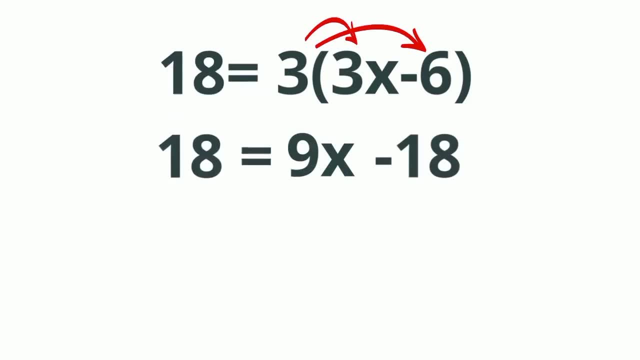 I'll bring down the other 18.. Now what I need to do is I can isolate the 9x by adding 18 to both sides. When I do this, bring down the 9x and 18 plus 18 is 36.. Now I can undo the multiplication. 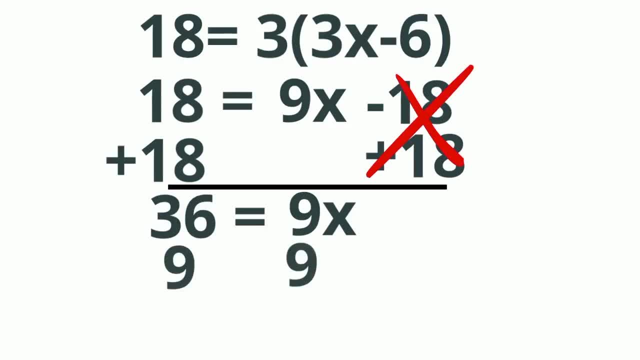 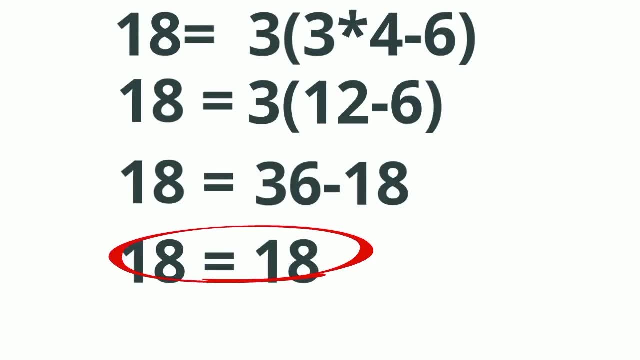 of 9x by dividing by 9, and when I do this, I get x equals 4.. And when I do this, I get x equals 4.. I plug it into the original equation. it does work out, it's correct. Next, I have 10, and, in parentheses: 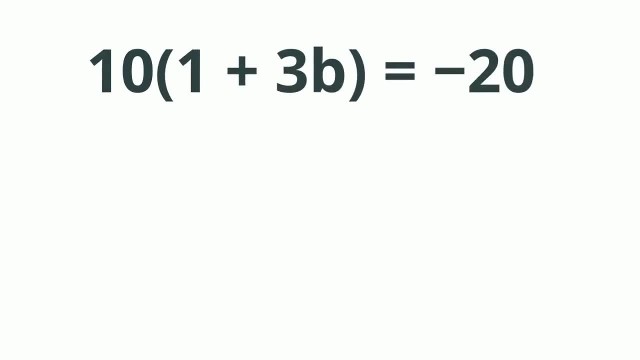 I have. 1 plus 3b equals negative 20.. I'm going to deal with the parentheses first, so I will distribute the 10. so that's 10 times 1 is 10. 10 times 3b is 30b, equals negative 20.. Now what I'd. 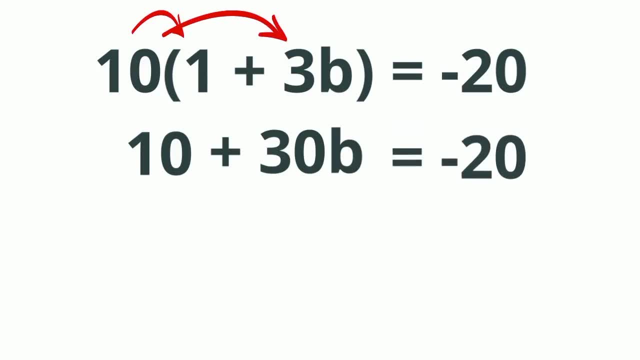 like to do is get the constants on one side, so I will subtract 10 from both sides. When I do this, the 30b comes down negative 20, and negative 10 is a negative 30. Now I will undo the multiplication of 30b, divide each side by 30b, and that equals b, equals negative 1 and you can see when I plug it. 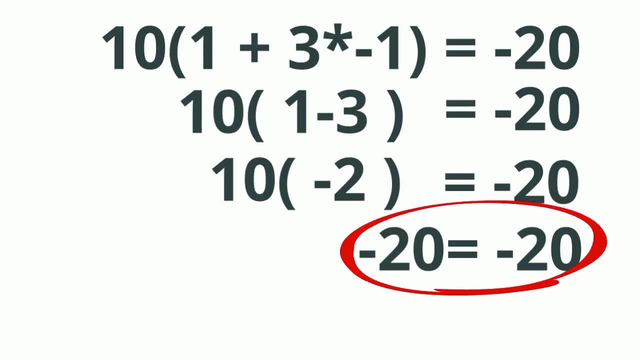 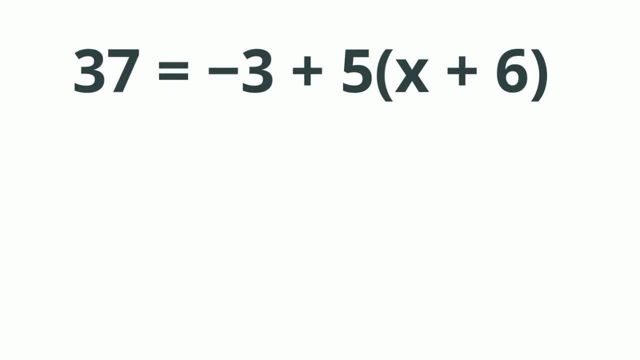 into the original equation. it is correct. And our last problem: 37 equals negative 3 plus 5, in parentheses, x plus 6.. So what I will do first is distribute the 5.. So 5 times x is 5x. 5 times 6 is 30.. Bring everything down Now. what I can do is combine. 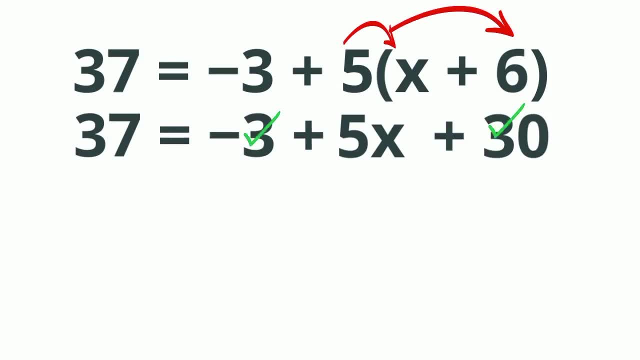 like terms. so I will combine 30 and negative 3 to give me 27.. Bring everything else down Now to isolate the 5x. I'm going to do the same thing. I'm going to do the same thing again. I will subtract 27 from both sides. When I do this, the 27 cancels. Bring down the 5x equals 10. 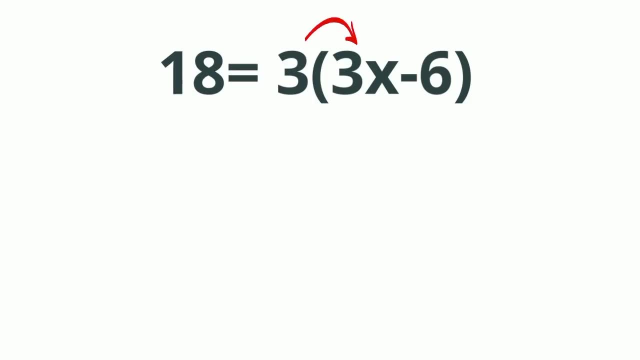 other. But first I need to distribute the three. that's on the outside, because I have parentheses and I'm going to deal with these first. Three times 3x is 9x and 3 times a negative 6 is negative 18.. I'll bring down the other 18.. Now what I need to do is I can isolate the 9x by: 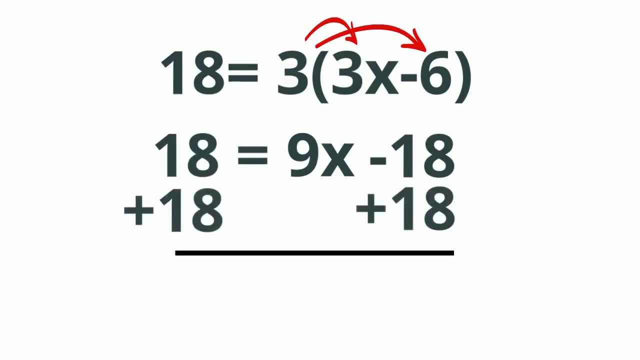 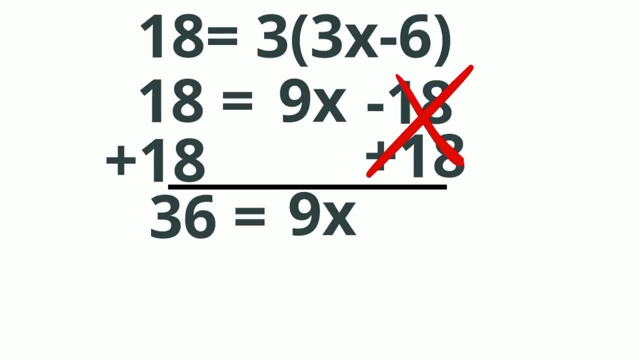 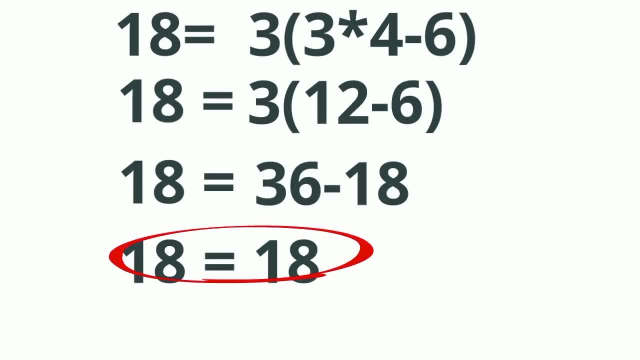 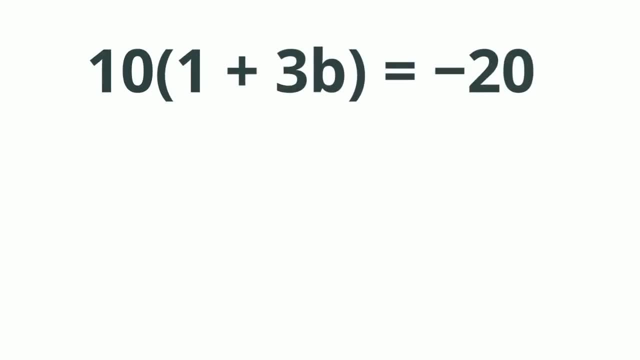 I plug it into the original equation. it does work out. It's correct. Next I have 10 and in parentheses I have: 1 plus 3b equals negative 20.. I'm going to deal with the parentheses first, so I will distribute the 10.. So that's: 10 times 1 is 10.. 10 times 3b is 30b, equals negative 20.. Now what I'd 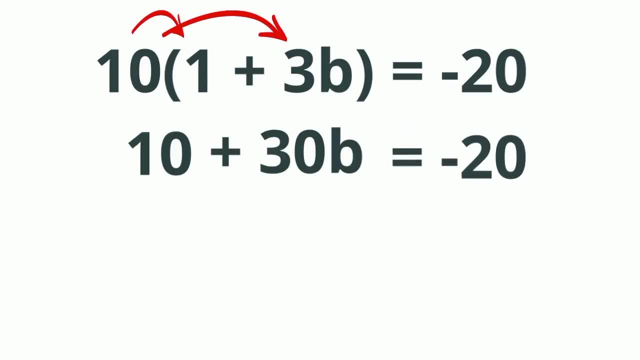 like to do is get the constants on one side, so I will subtract 10 from both sides. When I do this, the 30b comes down. Negative 20 and negative 10 is a negative 30. Now I will undo the multiplication of 30b, Divide each side by 30b, and that equals b, equals negative 1 and you can see when I plug. 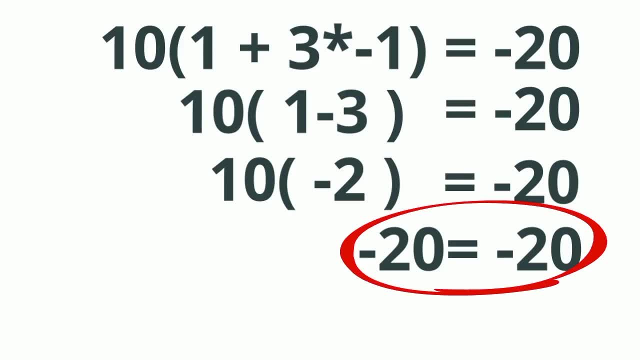 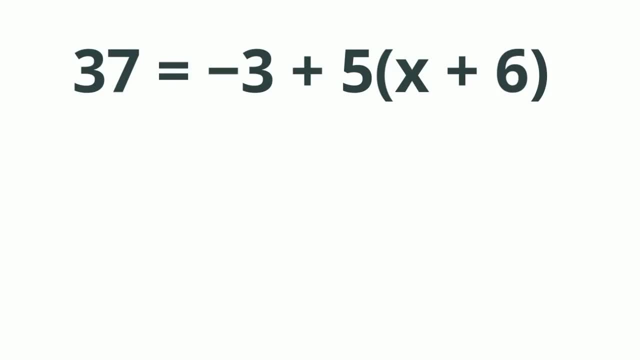 it into the original equation. it is correct. And our last problem: 37 equals negative 3 plus 5, in parentheses, x plus 6.. So what I will do first is distribute the 5.. So 5 times x is 5x. 5 times 6 is 30.. Bring everything down Now. what I can do is combine. 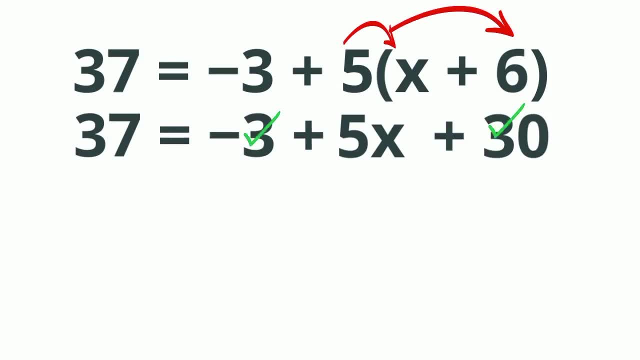 like terms. So I will combine 30 and negative 3 to give me 27.. Bring everything else down Now to isolate the 5x. I will subtract 27 from both sides. When I do this, the 27 cancels. Bring down the 5x equals 10.